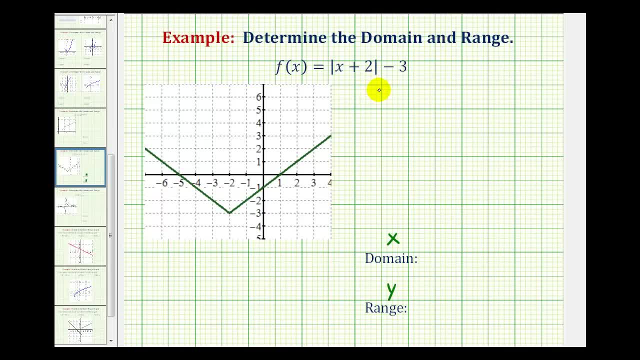 Let's start by analyzing the graph. So the first step would be to either make a t-table or use technology to create the graph provided here. Once we have the graph, we can analyze the behavior of the function horizontally and vertically to help determine the domain and the range. 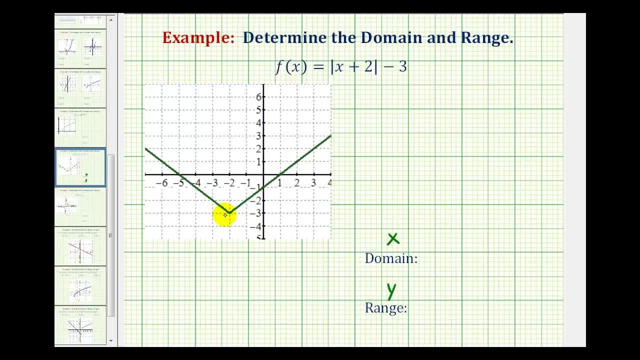 What I mean by that is to determine the domain. if we were to project this function onto the x-axis, notice how it would include the entire x-axis. Another way to think of this is: the graph continues to the right and continues to the left indefinitely, without any holes or breaks. 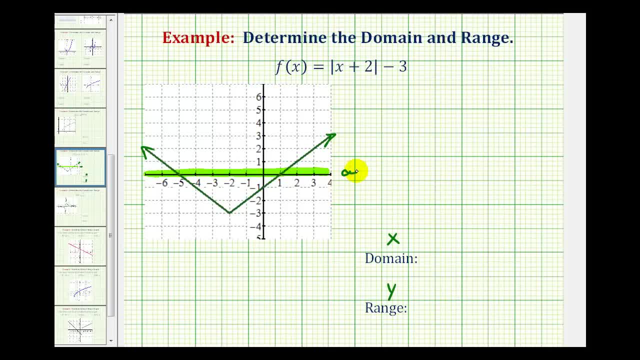 So the domain approaches positive infinity to the right and negative infinity to the left. Therefore, the domain of this function would be all real numbers. Or, if we wanted to use interval notation, we could use the interval from negative infinity to positive infinity. Now to determine the range, we would have to project the graph onto the y-axis or determine how the graph behaves vertically. 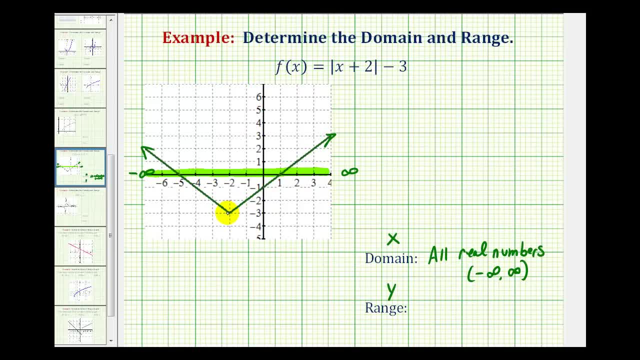 Notice how the lowest point on the graph is this point here, with a y value of negative three. And then from here, of course, the graph is moving to the right and left very quickly, but notice how it's also moving upward. So if we projected this graph onto the y-axis, 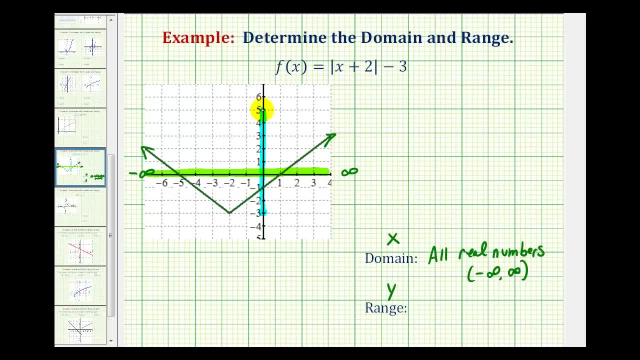 it would actually approach positive infinity along the y-axis, Which means the range would be from negative three to positive infinity, and it does include negative three. So we can say the range is greater than or equal to negative three Or, using interval notation, it would be the interval from negative three to infinity. 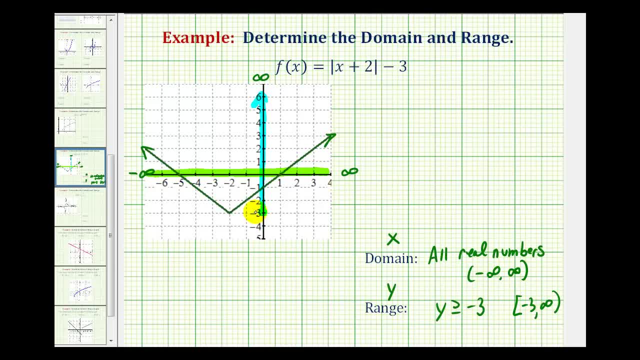 And it's closed on negative three, because it does include negative three. Now, if we didn't want to make a graph and we knew a lot about the properties of the absolute value function, we could use reasoning to determine the domain and range. What I mean by that is we could think to ourselves. 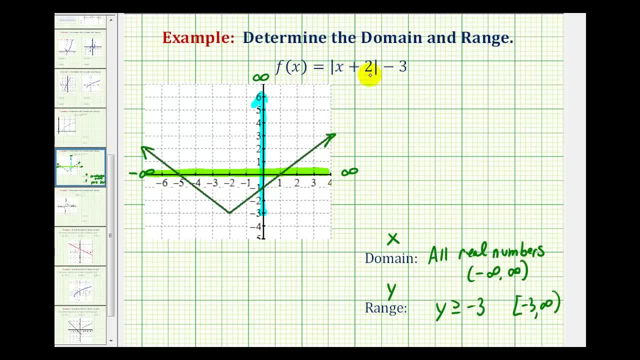 what are the possible values of x that we could use to substitute in here and then evaluate the function? And the answer is: we could use any real number here, add two to it, take the absolute value and then subtract three. And that's the reason why our domain is all real numbers.